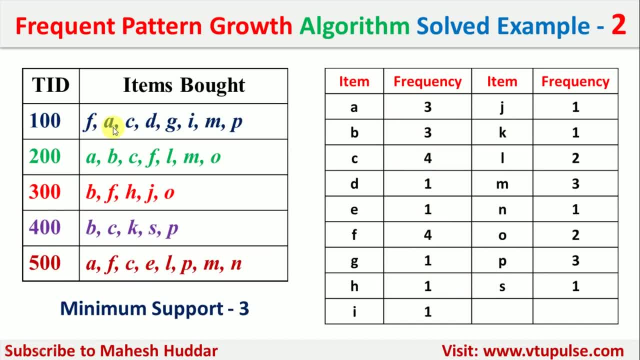 For example, A is appearing in the first transaction, It is appearing in the second one, It is appearing in the fifth transaction. So the number of times A is appearing is three here. Similarly B. B is not present in the first one. B is present in second, third and fourth one. So the frequency of B is three. Similarly the frequency of C is it is appearing in first, second, fourth and fifth year. 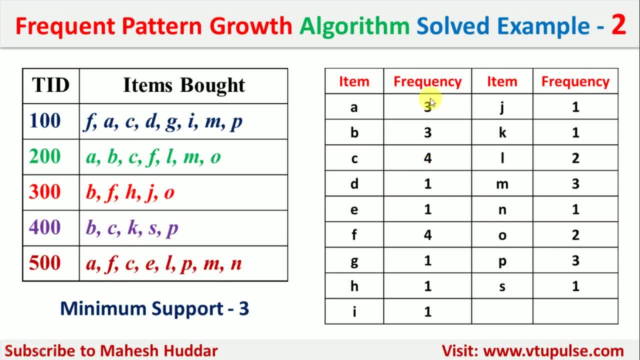 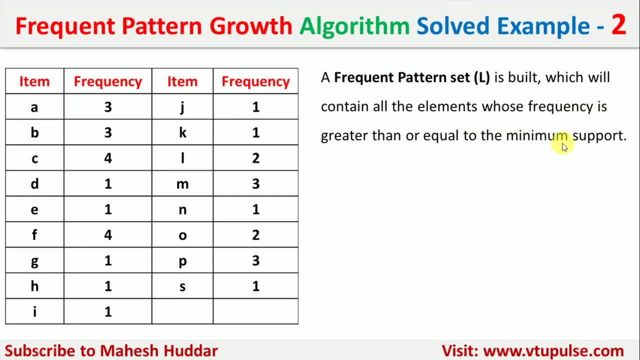 so it is appearing four times here. so we first we need to find the frequency of each item here. once we find the frequency of each item, next we need to build the frequent pattern set. frequent pattern set contains all the elements whose frequency is greater than or equal to. 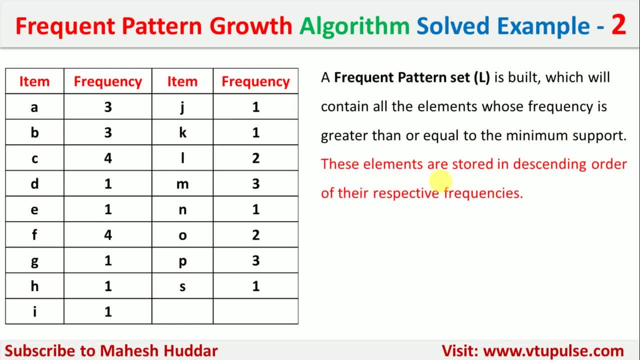 minimum support here. and one more thing is these elements are stored in the descending order of their respective frequencies. in this case, the minimum support given to us is three. hence we need to consider all those items whose frequency is three or more in this case. so the frequent pattern set, that is l, looks something like this: that is f4, c4, a3, b3, m3, p3. 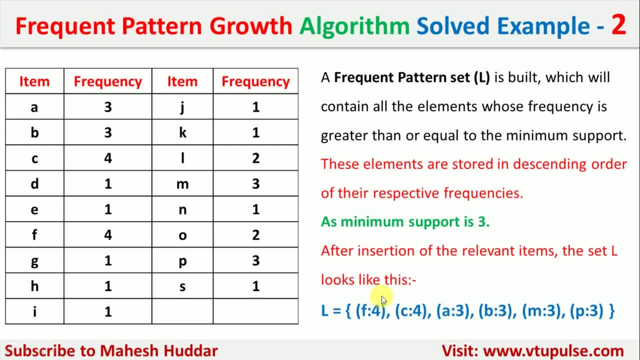 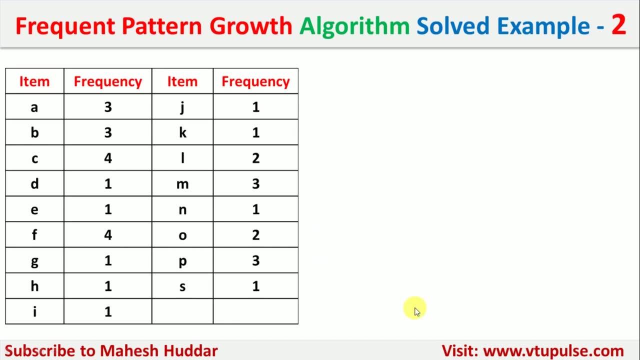 so this is the frequent pattern set, what we got by considering the minimum support three. here the first question comes in front of us is the frequency of f and c is four why i have written f first and then c second, if you just go back and see this particular 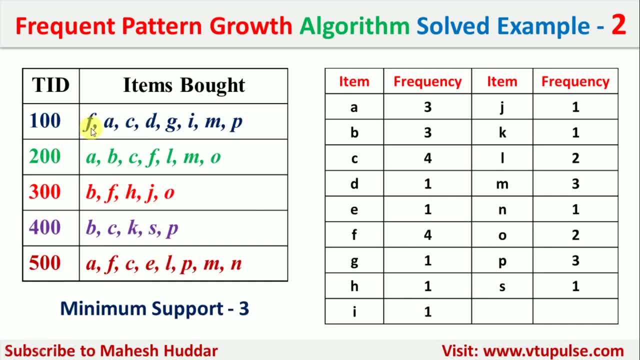 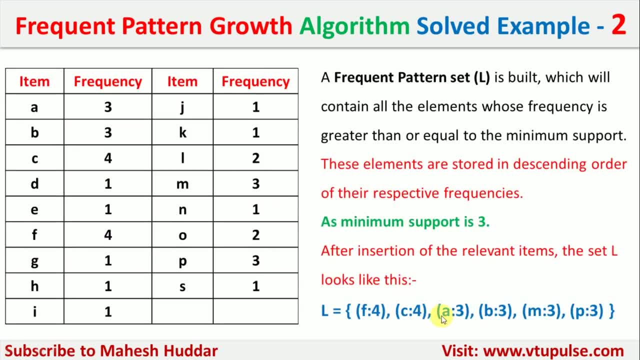 the order in which the items were bought. f was bought first and then c was bought. so that is reason i have written f first and then c first. the same thing is applicable for these also: a was bought first, then b, then m and then p here. because of this particular thing, we have listed these particular frequent patterns in this. 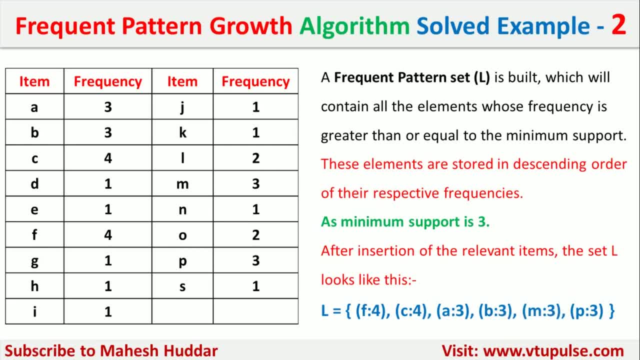 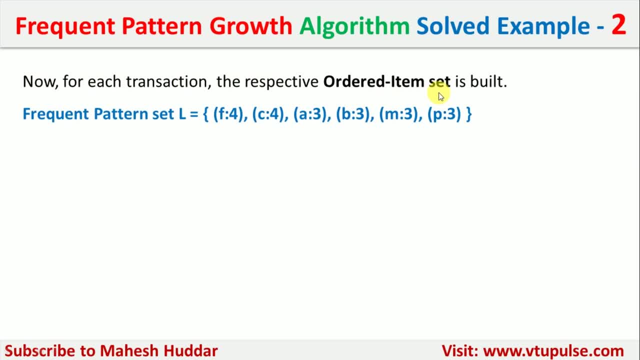 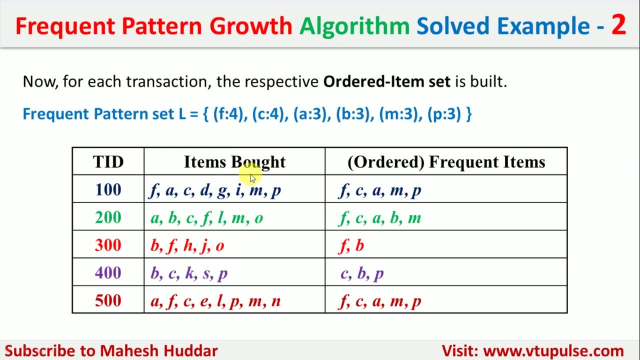 order here. once you build the frequent pattern set, that is l, we need to build ordered item set here. ordered item set is nothing but we have to cross check each of our transaction. if that particular item is present in the frequent pattern set, that will be present in the ordered item set here. so these are the items bought in the first transaction. 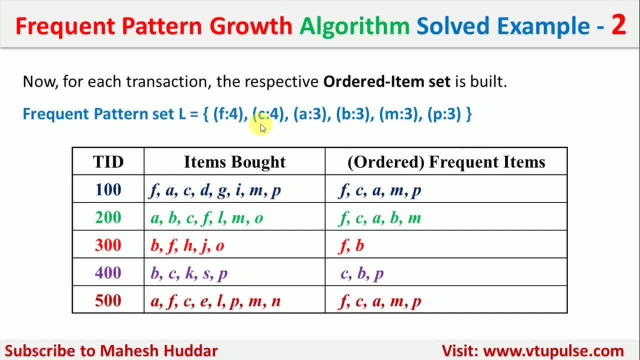 we will cross check whether they are present in the frequent pattern set or not. if they are present, we will list them in ordered item set. here f is present, a is present, c is present and m is present and p is present in the frequent pattern set. d, g and i are not present, hence we. 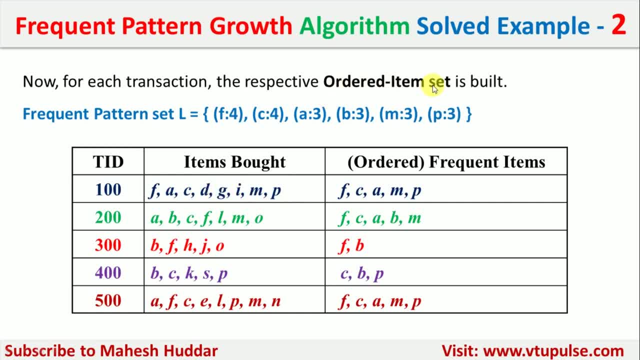 should not include those things in ordered item set. and one more thing we need to remember is we need to maintain this particular order here. so f will come first, a and c. both of them are present, but c will come first because the frequency of c is 4 and the frequency of a is 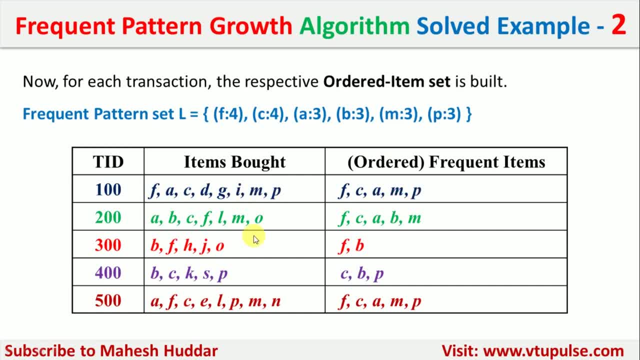 3 here. after that m and p will come over here. similarly, for the second transaction, a is present in the frequent pattern set, b is present, c is present, f is present, l is not present, m is present and o is not present here. now we need to check the frequency and then we need to. 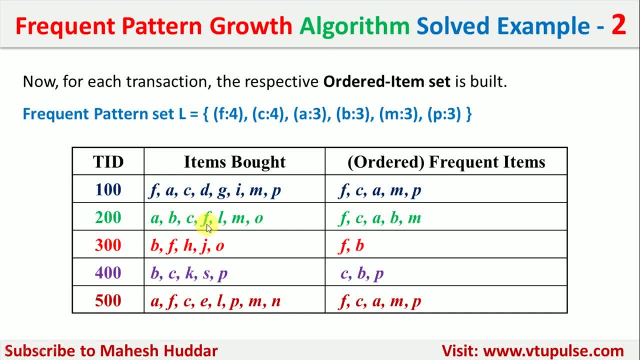 list it out in ordered item set, that is, f will come first and then c and then a, b and finally m. here the same procedure has to be repeated for the remaining three transactions so that we will get ordered item sets over here. so once we get these ordered item set, we need to build the tried. 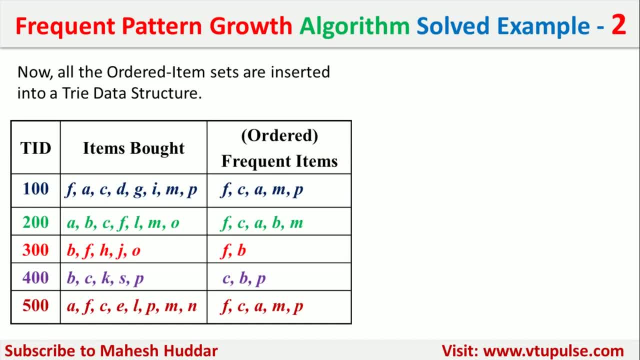 data structure from here onwards. so initially i will build this particular try data structure with only root node. this is the only node present. before i see any transactions here now i will consider the first transaction. in this first transaction, f, c, a, m, p are occurring in this particular order, so i will create the node for 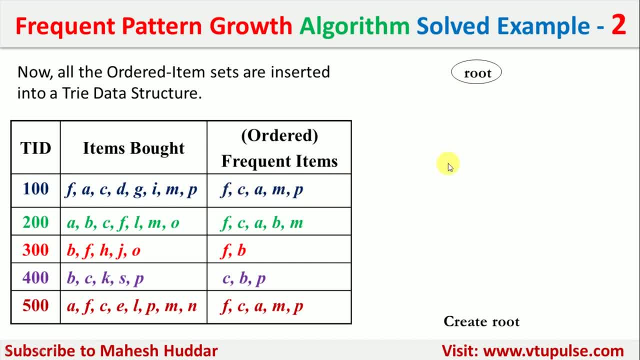 each and every item and then i will assign the frequency as one, because this is the first transaction order. so i will create the node for each and every item and then i will assign the, what we are seeing here. so we will get the first node as f here, that is f1, c1, a1, m1 and p1 here. 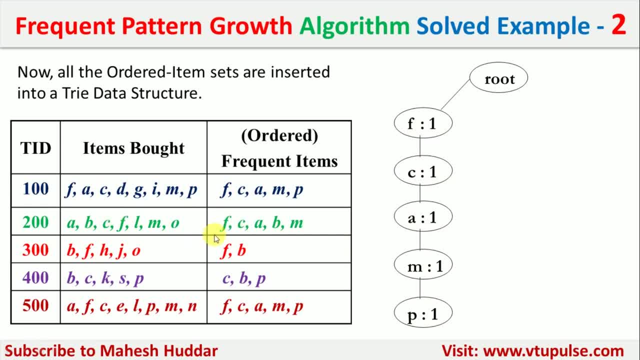 the next transaction is 200 and its frequent or the ordered items are f, c, a, b, m here. now again we will start traversing from root. we have f here, so f will be incremented by 1. that is the frequency of f i am saying. it will become 2. c will be incremented by 1. it will become 2. 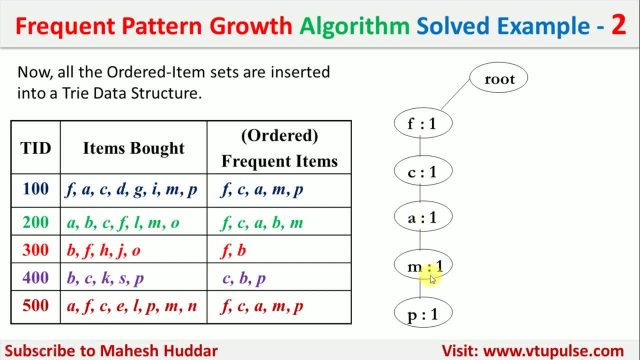 a will be incremented by 1. it will become 2 from here onwards. we are expecting b here, so b is not present. so we will create a branch here and it will become b1 and then m1 over here. so this is how actually the tri data structure looks like. after seeing the second transaction now considering: 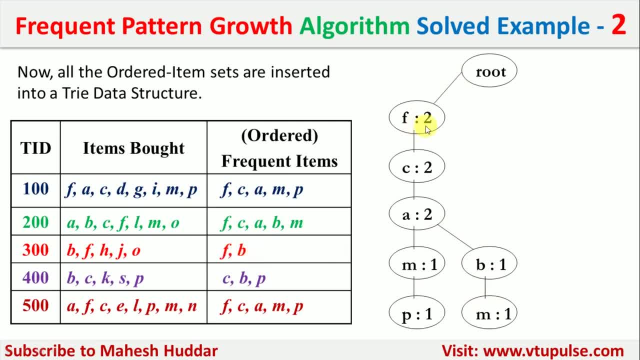 the third transaction. it looks like fb here, so the frequency of f will be incremented by 1. it will become 3 here. the next one we are expecting b. b is not present here, so b will come over here, so it will become b1 in this case. next one is c, b, p, so from root, if we start traversing, we have f here, so we don't. 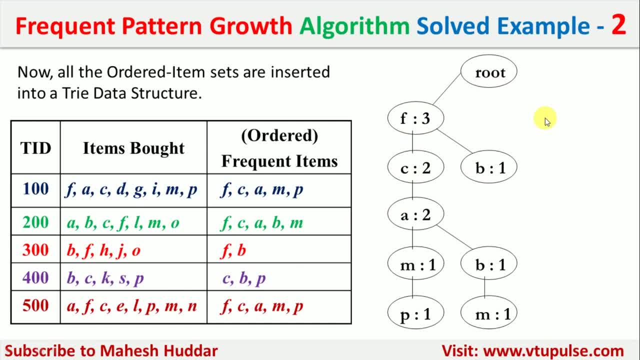 have c first, we will create a node with c as, and the frequency is 1, and then b and then p here. so this is the next path here. finally, if i see this, f, c, a, m, p- we will get something like this: f frequency will be incremented by 1, it will become 4, c, 3, a3, m2 and then it will become p2 here. 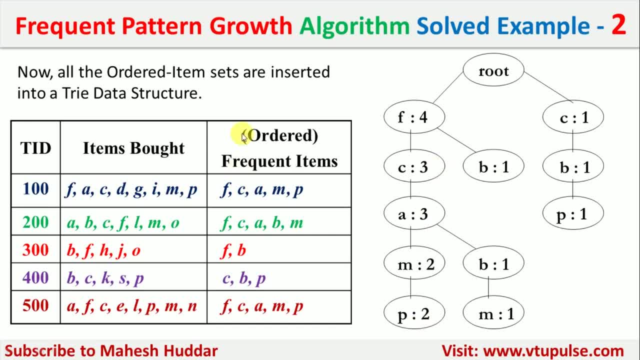 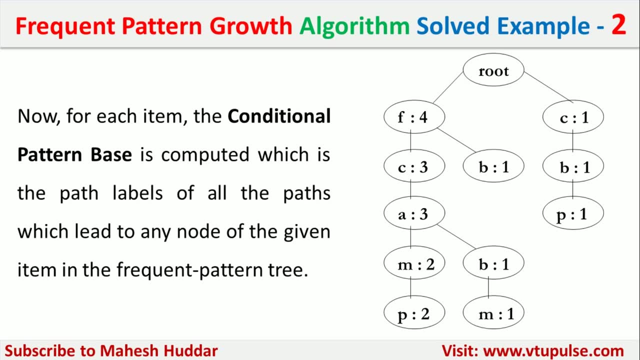 so this is the final tri data structure, once we see all the transactions here, and it is also called as a frequent pattern tree here. once you build the frequent pattern tree, next thing is to build the conditional pattern base, which is computed by traverse each of this particular path, and then the leaf nodes will become the items in this case. 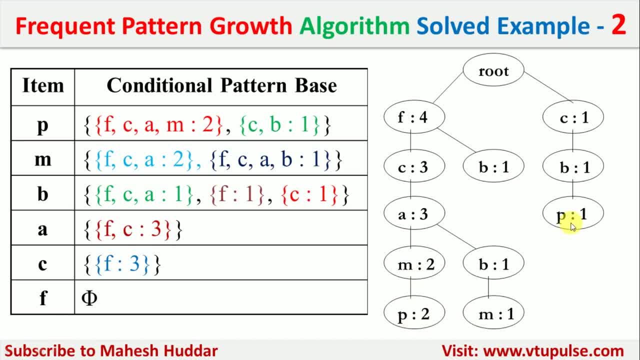 for this particular p. p is present two times as the leaf node, so we will get two. what we can say that the conditional pattern basis for p. for this one it will look something like this: f, c, a, m, and then the frequency is two here for p, one more we have that is a, c, b, colon one, because the 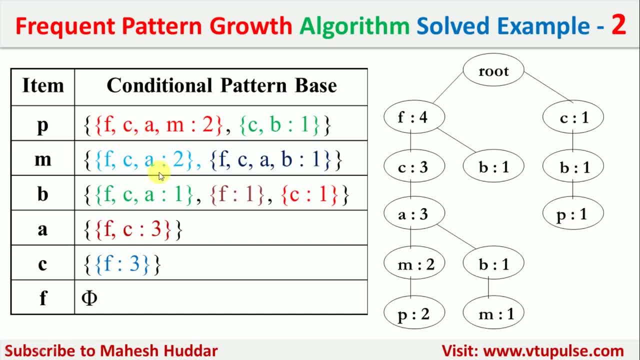 frequencies: one for this particular p here. similarly for the second one, that is m. usually we go from bottom to top. so we have considered p here. next we will consider what is that called as m here for m we have two paths again: f c a. the frequency of m is two: f c- a. 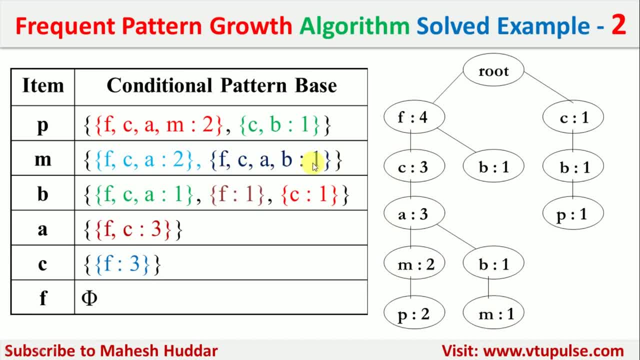 b, b and frequency of m is 1. so that is what i have written here. now we have done with p, we have done with m here. next we will consider b. so if i consider b, f, c, a frequency of b is 1. so that is the one conditional pattern base i will get. second one is f: 1, because we have only this, this 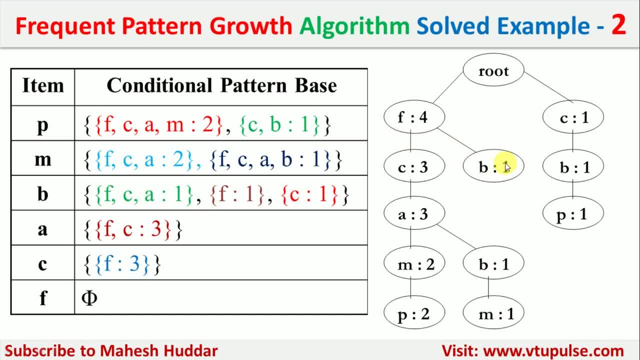 is the path here, and one more is we have b here, so that is nothing but c, colon 1. this is the path here. next we we have a here, so for a, this is the only path we have, that is f, c, the colon 3, because 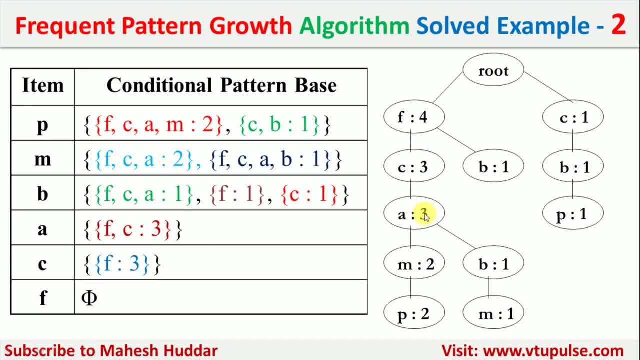 the frequency of a is the 3 here, and for c, this is the only path. we have f, colon 3, because the frequency of c is equal to 3. for f there is nothing. no path exists. so we write: what is that called as null for f here? so we have to write the conditional pattern base. 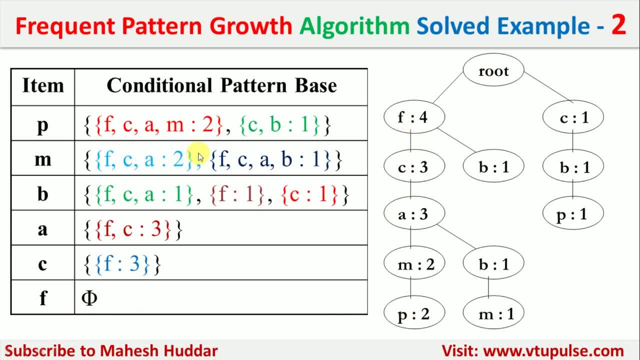 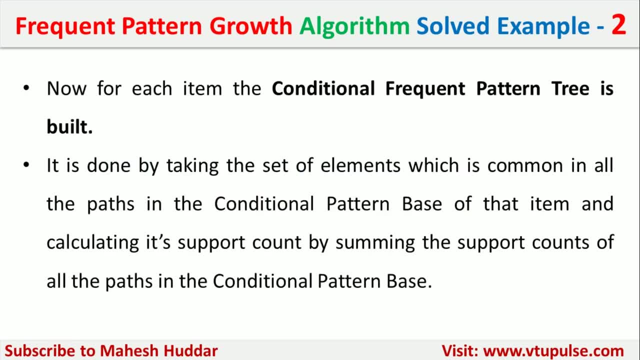 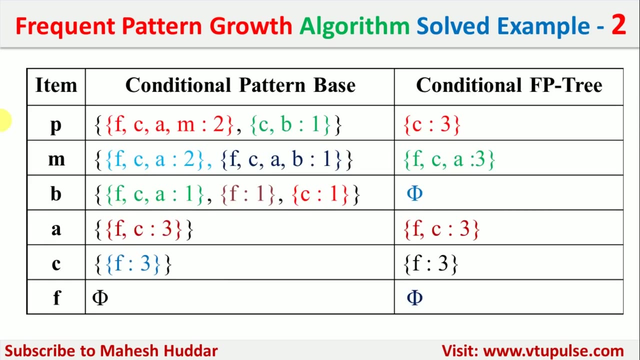 starting from bottom to top, and they look something like this: once you build the conditional pattern base, the next step is to build the conditional pattern frequent pattern tree. it is done by taking a set of elements which is common in all the paths in conditional pattern base. that is nothing, but you can see here if you consider the first one that is conditional. 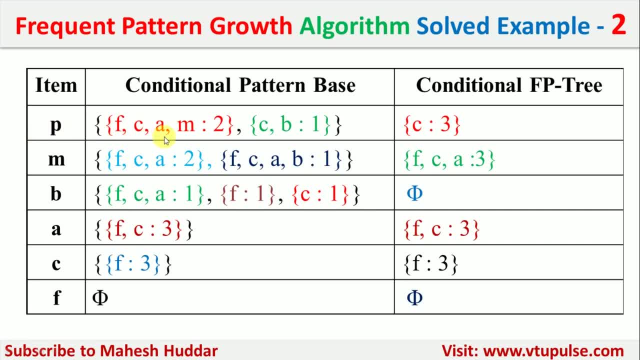 frequent pattern tree and then you can see that it is common in all the paths in conditional pattern tree for p is. we need to consider these two paths and then we need to check the common elements between these two. c is the only common element, so c will come here, and then we need to add the. 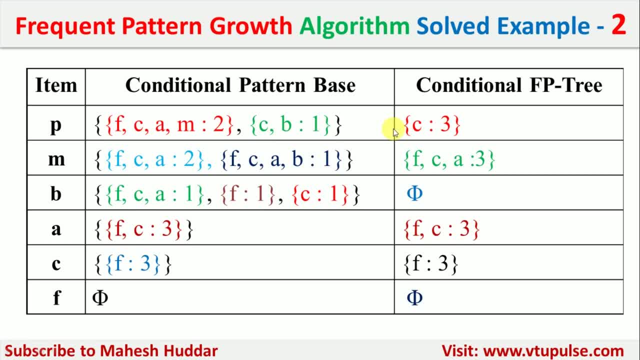 frequency of these two conditional pattern bases. so 2 plus 1, that is nothing but 3 here. now, considering m, between these two, f is common, c is common and a is common. so we will write those things and 2 plus 1, that is the frequency, will become 3 here for b. if i consider these three, 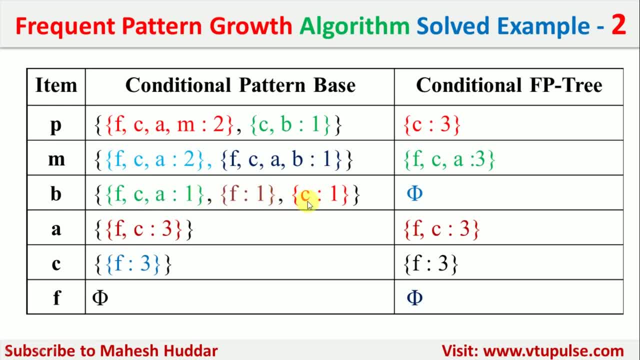 there is. none of the elements are common here, so we don't get any conditional frequent pattern tree here. for a, we have only one conditional pattern base, so it will be retained as it is. for c also, we have only one conditional pattern base. it will be retained as it is. for f, we 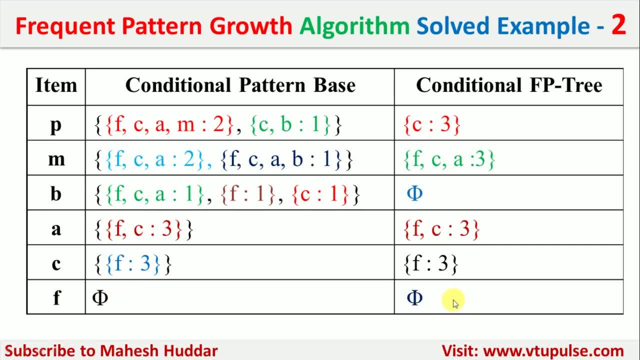 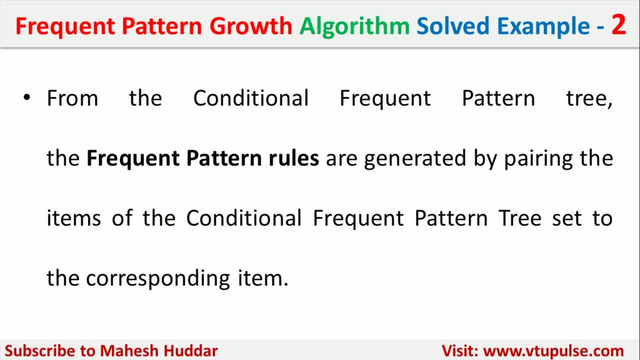 don't have any conditional pattern base, so conditional frequent pattern tree contains nothing here. now from this particular conditional pattern tree we will get only one conditional pattern pattern tree. we need to build the frequent pattern rules. They will be built by pairing the items in the conditional frequent pattern tree and the corresponding item here, That is, you can see here. 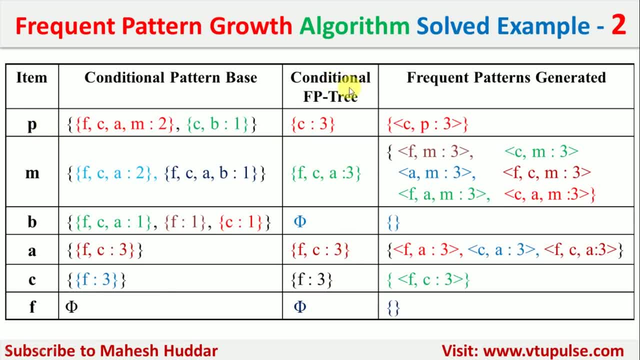 the item is P and the conditional pattern frequent pattern tree contains C3. So we need to combine these two things or pair these two things, and then we need to write the frequent pattern rule here. So there is only one possibility exists. that is nothing but CP and the frequency is 3 here 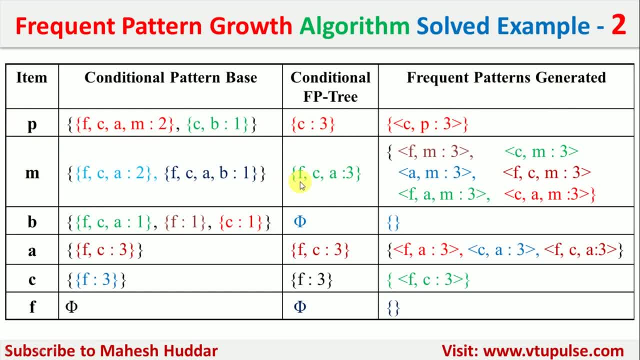 But when it comes to second one, that is M, there are multiple possibilities. are there that is nothing but FM. that is the first one and the frequency is 3, always because we have 3 here. CM is the second possibility, AM is the third possibility. 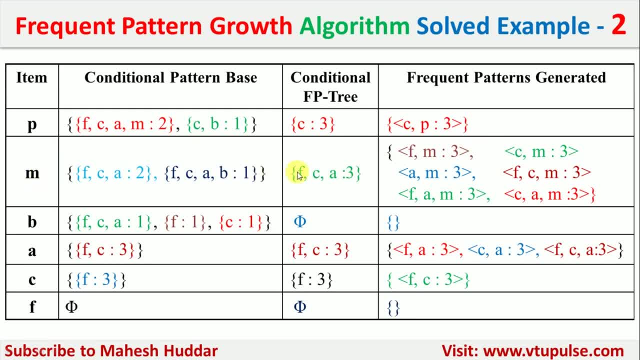 Next possibility is FM- c m, another possibility is f a m and the last possibility is c a m here. so totally we will get six possibilities here. for this one we don't get any possibility, that is for b, because we have null in the conditional frequent pattern tree. the next one contains f- c here. so the possibilities: 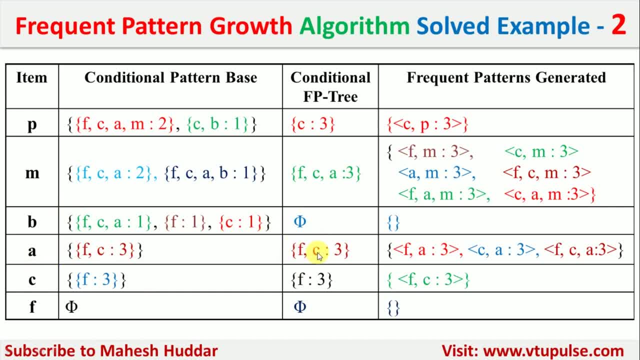 are f a 3, c a 3, f, c a 3. those are the three possibilities. considering this one, f, c 3 is the one more possibility for c. for f, we don't have any possibilities in this case. so these are nothing but the frequent pattern rules, what we have generated using frequent pattern growth.